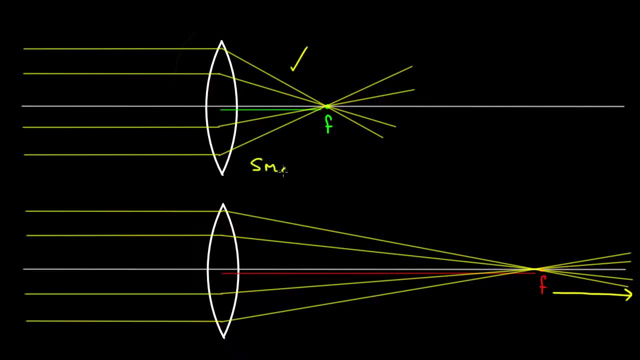 So this is a little weird, but small focal length means a powerful lens. So rather than talk about focal length, optometrists and ophthalmologists often talk about lens power. So the lens power is just defined to be solar. Solar has no such power. 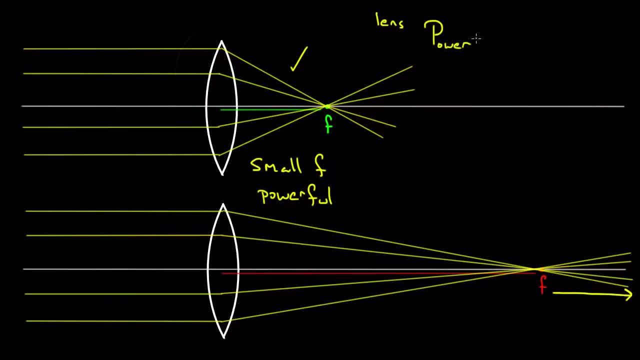 So to us. so to us, it's just somebody's wish defined to be. this isn't power like joules per second. this is lens. power is defined to be one over the focal length, and so, if you're using SI units, 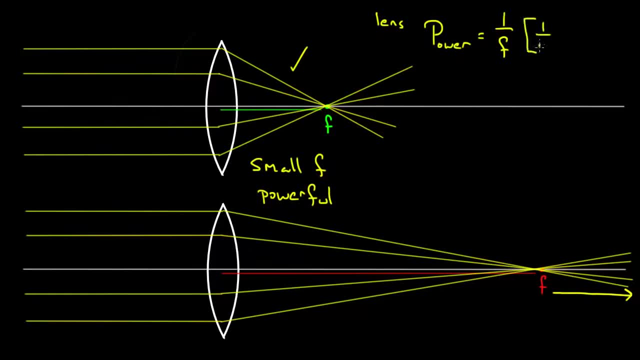 we'd have one over meters and that's given a special name That's called diopters. So a one over a meter is called a diopter and this is what optometrists and ophthalmologists use to measure lens power in. 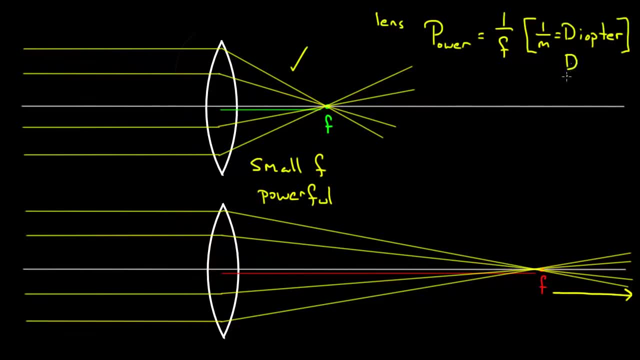 it's represented with a capital D. This makes a little more sense, because if your diopter measurement is large, that means powerful lens, and if your diopter measurement is small, that means not as powerful of a lens. and so, in other words, if this focal length up here 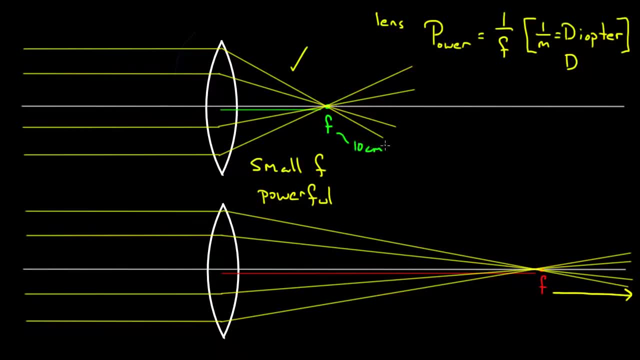 was 10 centimeters, well, I'd have to convert it to meters, so 10 centimeters is .1 meters. and then to get the power, the power for this lens would be one over the focal length in meters, so I'd have one over .1 meters. 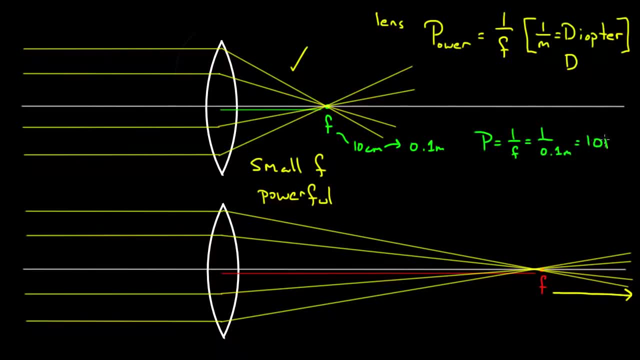 and that would mean this is 10,, a 10 diopter lens. It's supposed to be a D 10 diopter And down here, if this one was more like 50 centimeters, I'd say that the power is one over F. 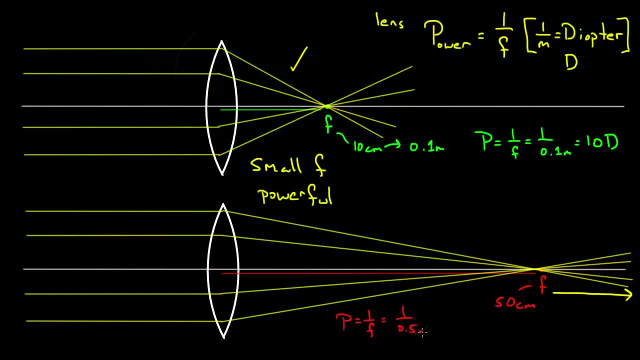 I gotta convert to meters, so one over .5 meters and I'd get two diopter or two, one over meters, so a diopter has you units of one over meters or meters to the negative one. Now I'm kind of lying a little bit. 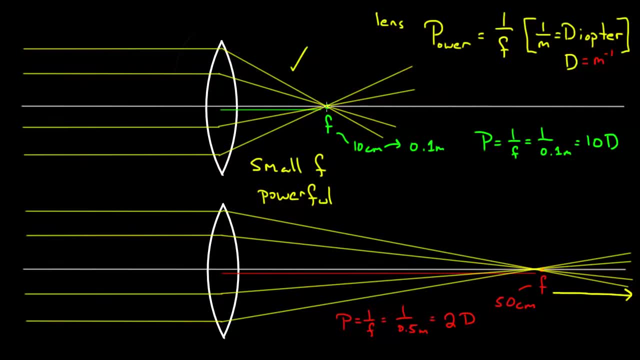 Spherical lenses don't actually send their light rays exactly through the focal point- not all of them. If you're sending parallel light rays like this through the whole face of the lens, some of them are gonna miss a little bit and it's called spherical aberration. 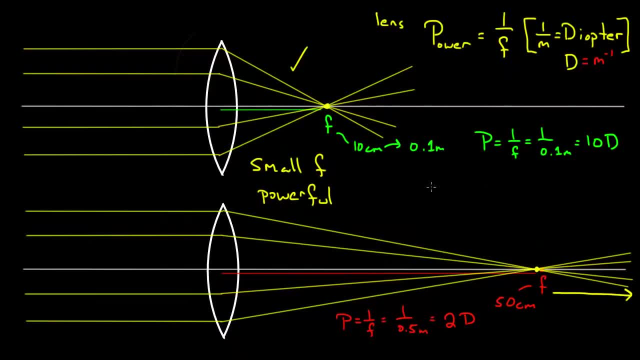 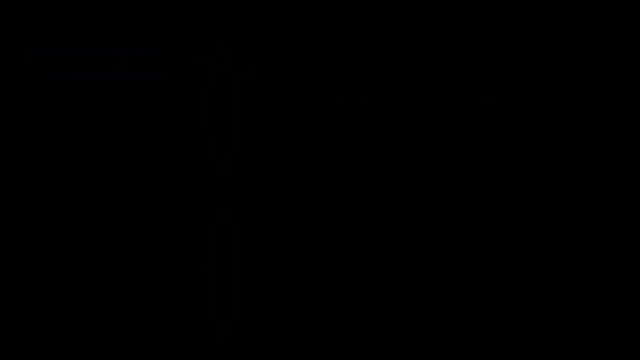 so another thing that you'd be interested in, if you're trying to craft precise lenses for a specific purpose, is the idea of spherical aberration. Let me show you what that's all about. so let me hide these. So what's supposed to happen? 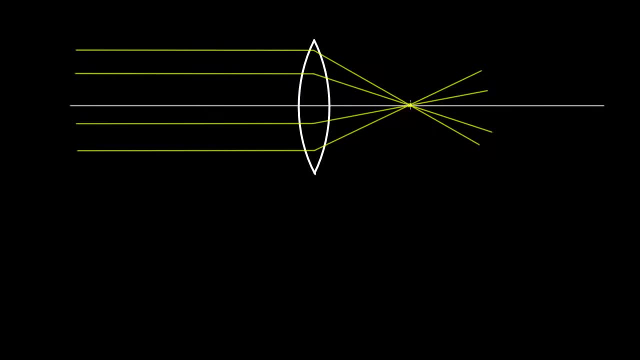 parallel light rays are supposed to get sent exactly through the focal point. Boom, right there. What actually happens is parallel light rays get sent, the ones on top get bent a little bit more and they might focus around this point, and the ones closer into the center of the lens. 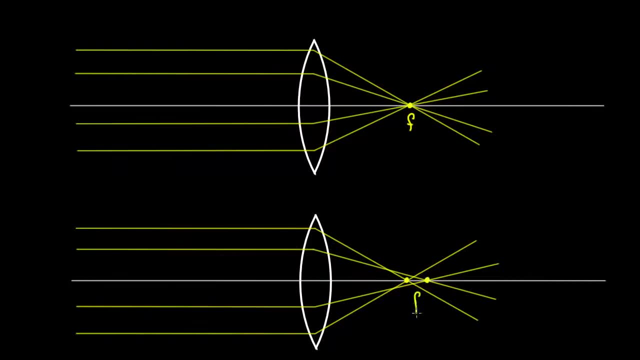 get sent over here, and so this spherical convex lens kind of focuses all the light to a point, but it creates a little bit of a blur here. so this is called spherical aberration and this is an inherent problem with spherical lenses. 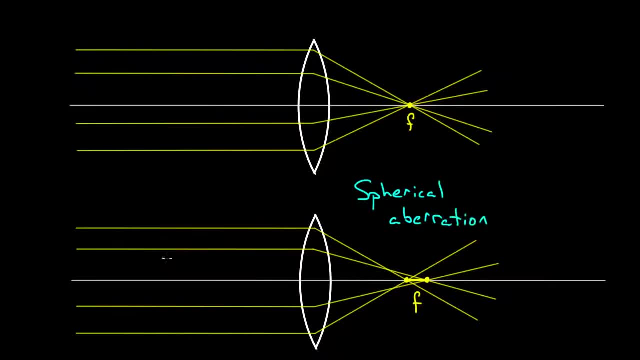 The light that gets sent through the top gets bent a little bit more than the light that gets sent more toward the middle, and so you've got this problem. This is a problem if you have a highly precise situation that you need to create an image for. 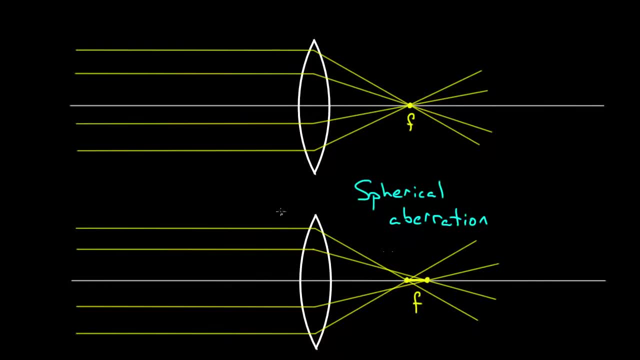 it might get a little bit blurry because of spherical aberration. So you might wonder why does this spherical aberration happen? It has to do with the fact that you know how we're always calling these thin lenses. You might wonder: why are we always calling them thin lenses? 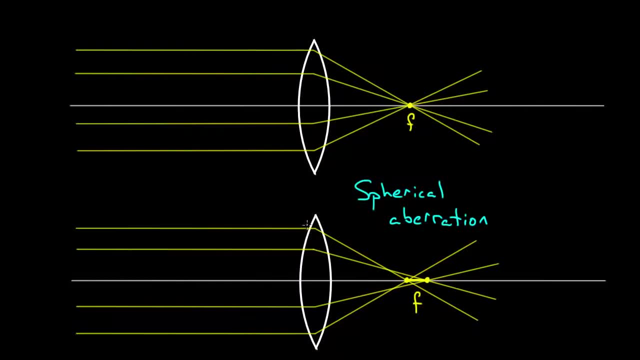 Why do they gotta be thin? It's because if they're thin, all these angles involved for these normal lines are gonna be small. and if the angles are small, that's a good thing, because in physics, physicists love this one. Here's a trick we like playing. 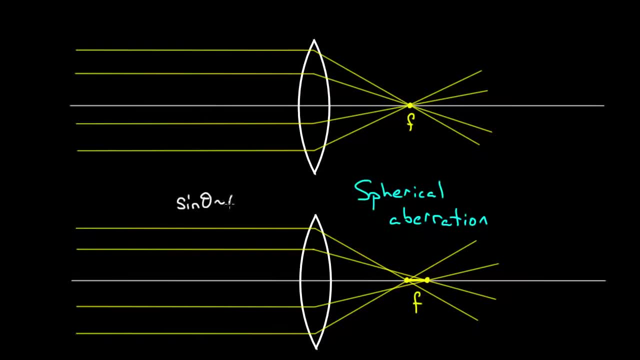 Sine theta for small angles is approximately just theta, and so there's all kinds of approximations here that you can use if the lenses are thin and you get that they all go basically through the focal point, but there's a difference between. 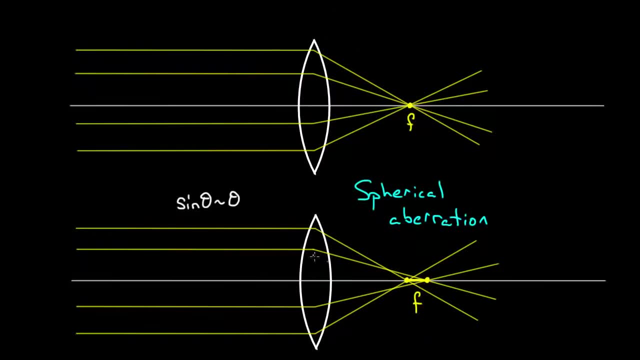 basically going through the focal point and exactly going through the focal point. and the farther you get up here, the larger this angle's gonna be, the more deviation you're gonna get. It's just a problem inherent to this spherical lens. The problem is it's easy to make spherical lenses. 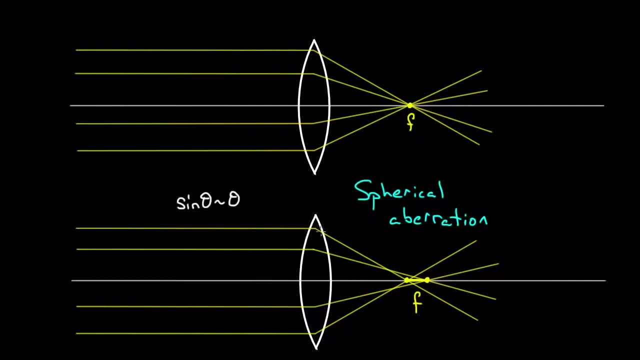 I mean, it's easy to make a perfectly spherical shape. If you wanted to make one that did send them exactly through the center, it'd be harder to do. You'd have to pick a different shape, because spheres just don't cut it in that case. 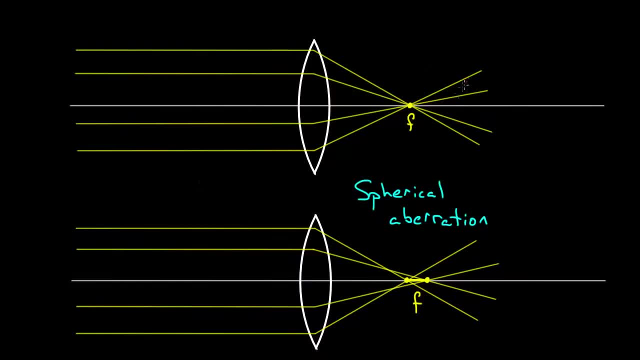 Spherical aberration's not even the only type of aberration. There's other kinds of aberration. One of them is chromatic aberration and, as the name suggests, this has to do with color and remember dispersion with lenses or any material. 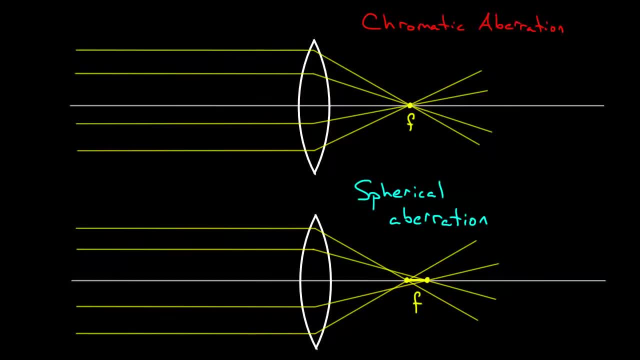 dispersion says that some colors bend more than others, so some colors experience a higher index of refraction. Red, it turns out, experiences a smaller index of refraction. so these red rays would get sent. they'd get bent a little bit less than yellow. 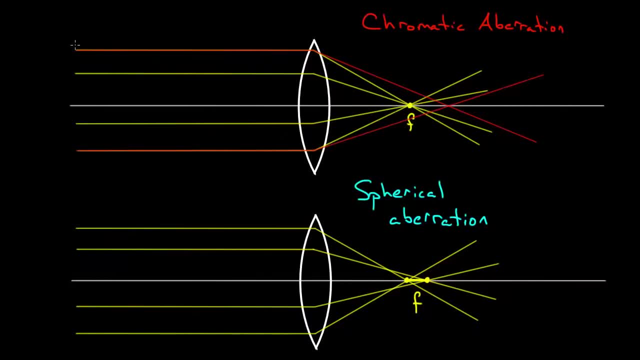 so they might meet up there. and blue rays: blue gets bent more. Higher frequency light gets bent more, and so you'd get these colors separating. so this is another way of looking at it, Another problem with spherical lenses or any type of lens. 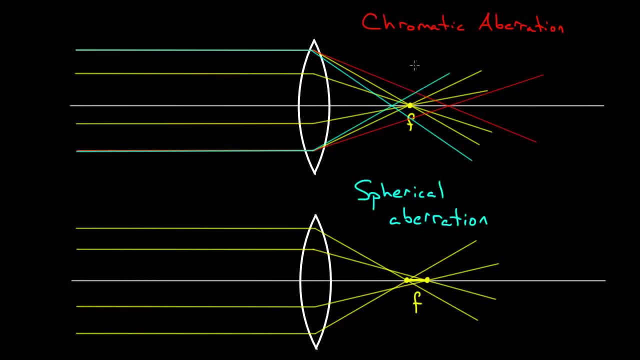 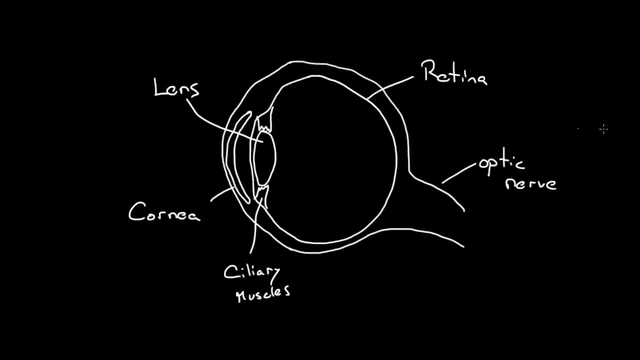 is, you might get some sort of chromatic aberration. so these are things to look out for if you're trying to create a precise optical instrument. One of the most precise optical instruments is the human eye, and in the human eye you have a lot of parts. 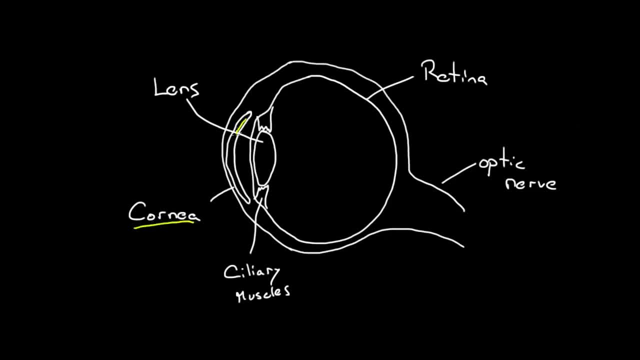 Up front you've got the cornea. This acts like the main lens. This is the front lens here. This does most of the bending of the light. but you've also got this inner lens- that's just called the lens, and this inner lens is more adjustable. 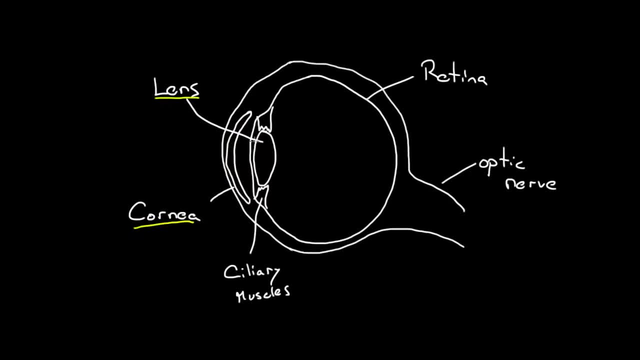 This can sort of make fine adjustments to what you're looking at. If you're depending on how close something is to your eye, this can adjust and these ciliary muscles are muscles that can exert a force on this lens and can change the shape of it. 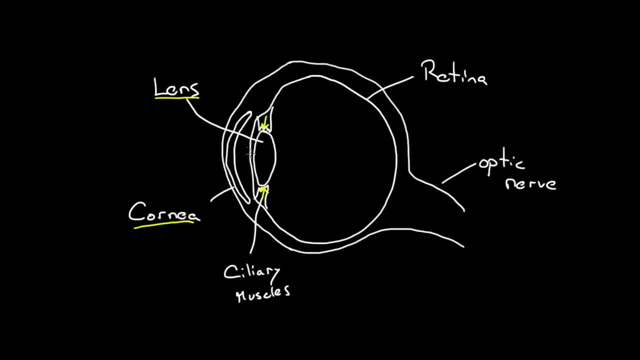 This is bendable. This inner lens is bendable and, depending on what distance away the object is, these ciliary muscles can change the shape of this lens to make sure that the image is formed right on here. to make sure that the image is formed right on here. 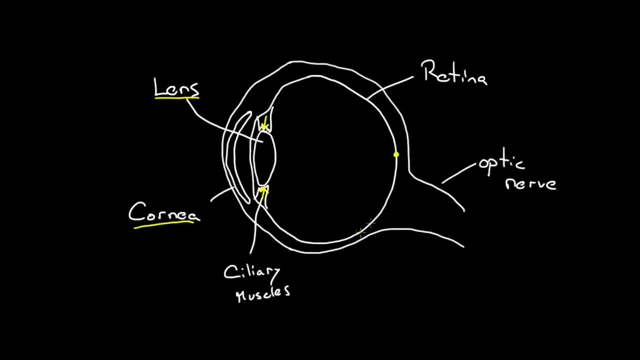 On your retina. this back wall acts as the screen of your eye and this is where you want the image to form. If you form a nice, clean, precise image on your retina, the optical nerve can take that information to your brain and you get a nice, clean image of whatever it is. 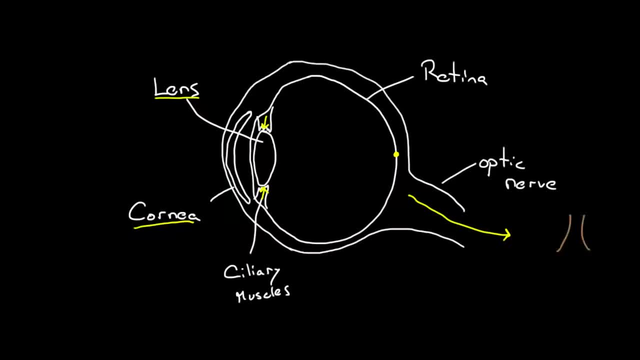 you're looking for. maybe it's a tree. Now, the weird thing is, so here's your tree, maybe you see this. but here's the weird thing: You've got this cornea and this inner lens are both convex, and if you're gonna see a real image, 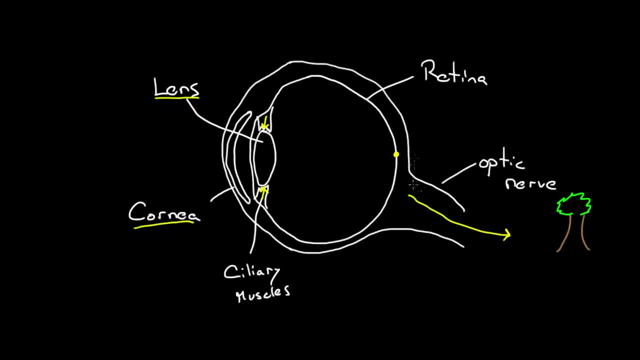 that's actually projected on a screen here. this is actually gonna be an upside down image. your tree image that forms actually on your retina is an upside down real image, so your optical nerve sends that information to your brain. somewhere in your brain it flips it over. 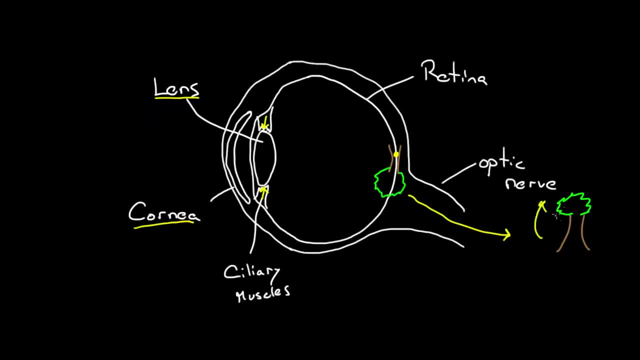 and then you get a clean image of a tree that's right side up, All right. so if you were looking at a far away tree- let's say the tree was really far away and these light rays were coming in basically parallel- you'd wanna make sure your cornea and your inner lens 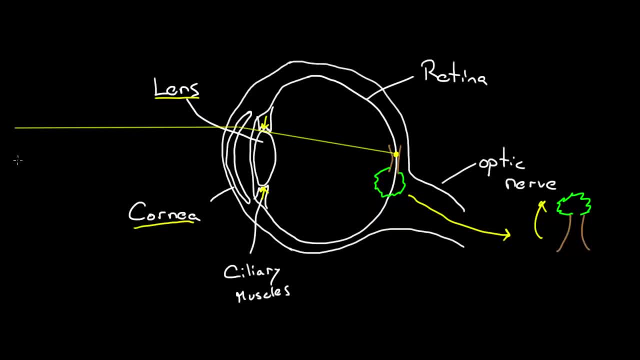 were able to focus these light rays from some point on the tree straight into the retina and you form a nice clean image at the retina. So that's good. let's say you're able to do that. just fine, you get a clean image of this tree. 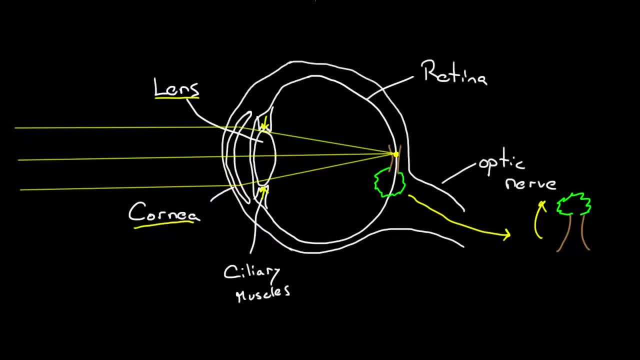 what if you got a little bit closer? Maybe you get a little closer and now the image isn't so clean. so you got this tree here. you're looking at a particular part of it. maybe you're looking at this part right here. 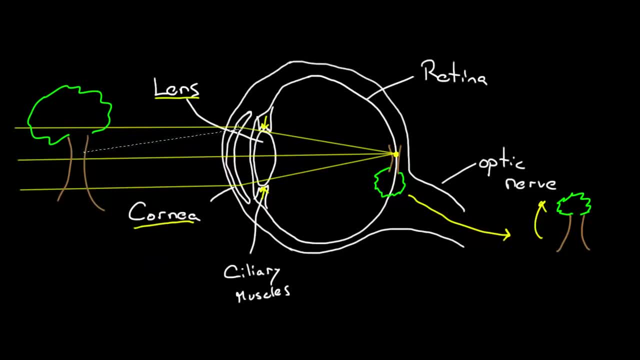 you're a little closer, this part comes in here. we're looking at light rays out of here. it's not gonna get bent as much. your ciliary muscles are gonna have to adjust, but maybe they can't cut it and this forms an image. 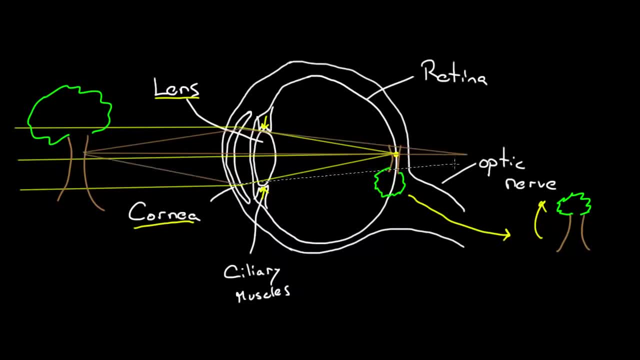 back here. but that's bad. that's bad because if you form an image behind your retina that's gonna be blurry. you're not gonna see the nice clean image here. you're gonna get this weird blurred out image. so your ciliary muscles. 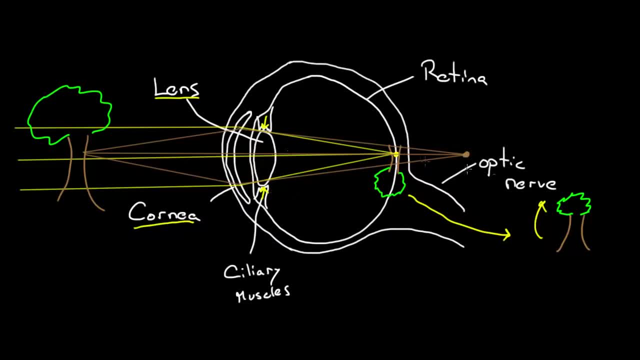 are gonna try to compensate, but maybe they can't. so this person might need glasses. this person: if they were able to see the far away tree, just fine, but things up close were hard for them to focus on. we'd call this person farsighted. so farsighted people. 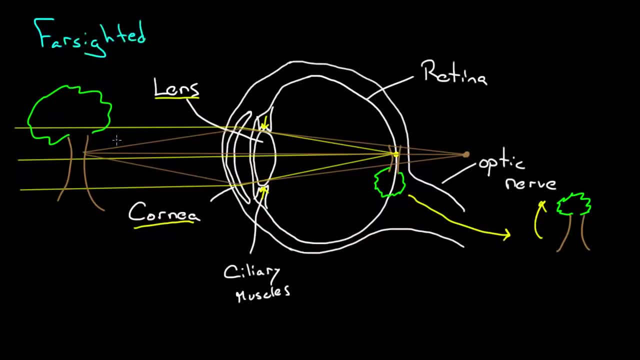 can see far away stuff, just fine, but when it's too close, they can't focus on it. so what do we do? we add another lens in here. we're gonna add a lens that tricks our eye. see our eye, this farsighted person. 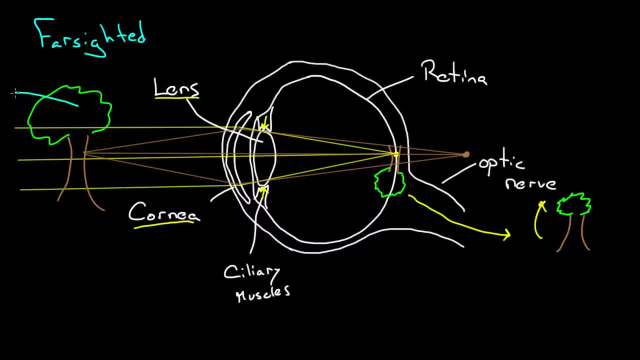 was good at seeing stuff far away, so I'm gonna try to take this tree, this object, I'm gonna try to make an image of it farther away. so how do I do that? I'm gonna prescribe this person a convex lens. 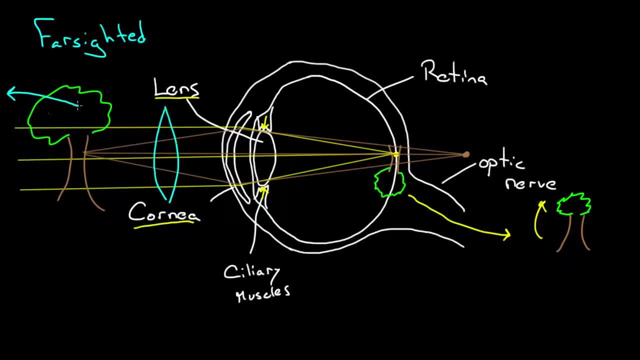 because the convex lens will create a virtual image of the tree at some farther away point. we trick our eye. now it can focus a little better. we can take this image and bring it up to our retina, get a nice clean image of the tree. so that's for a farsighted person. 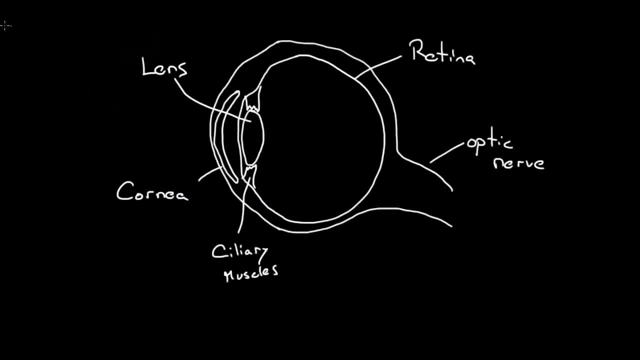 for a nearsighted person, let me get another image in here. nearsighted people can see stuff near just fine, and it's the far stuff that they have trouble with. so for a nearsighted person focusing on this tree up here: 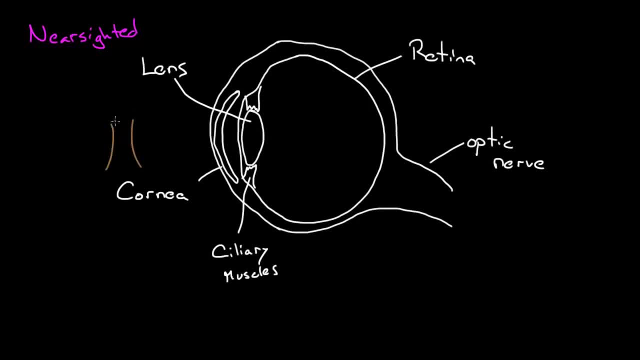 that's no problem. they can focus on this just fine, get a nice clean image of the tree right at the spot where it's supposed to be at at the retina, you get a nice clean image. but if you move the tree further away they'd have trouble. so we need to take 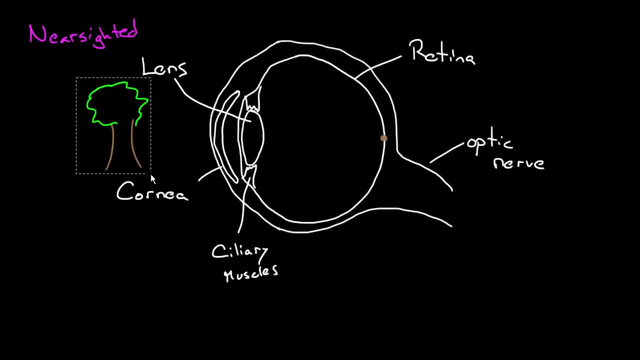 this tree. I'm gonna take it right here. so I'm gonna take this tree and I'm gonna move it farther away. now the eye has trouble seeing it, and so now the eye's gonna form an image. maybe the eye forms the image up here. that's not good. 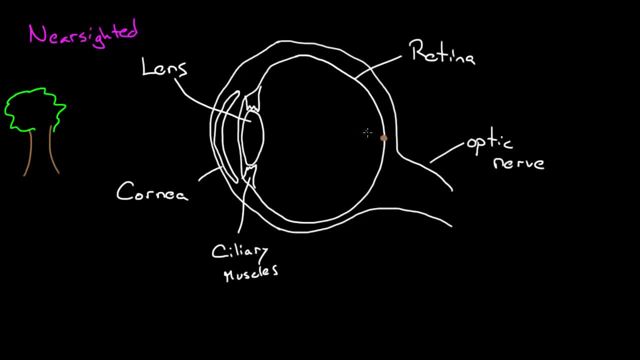 we need to bring this back over to this way, and so we'll have to prescribe a lens. this person was able to see near stuff, just fine. so again, we're gonna have to trick our eye. we take this object. we need a lens that makes our eye. 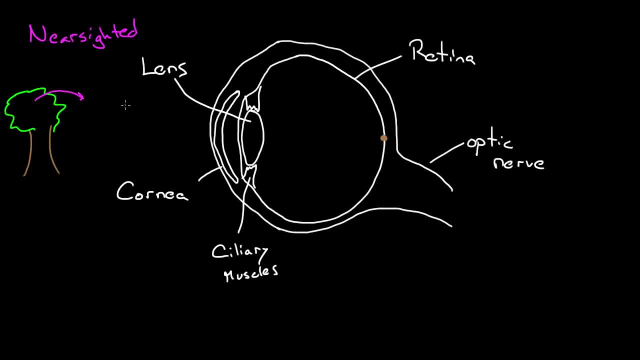 think that this object's closer than it is and we'll prescribe this person a diverging lens or a concave lens, and this lens is gonna make a virtual image of this tree that's a little bit closer than the actual object was. 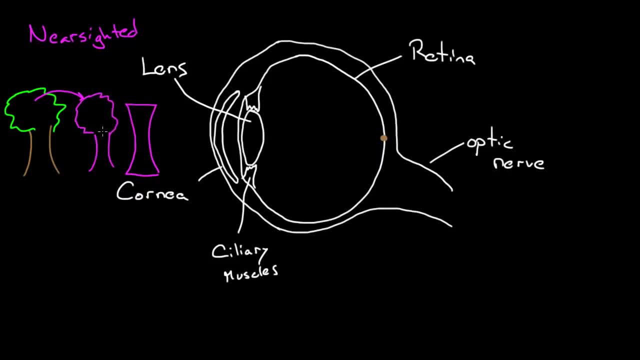 so now our light that comes in to our eye. once it gets to our eye- I'm neglecting a lot of bending going on here- we can actually get this light to focus right on our retina, which is what we wanted it to do.